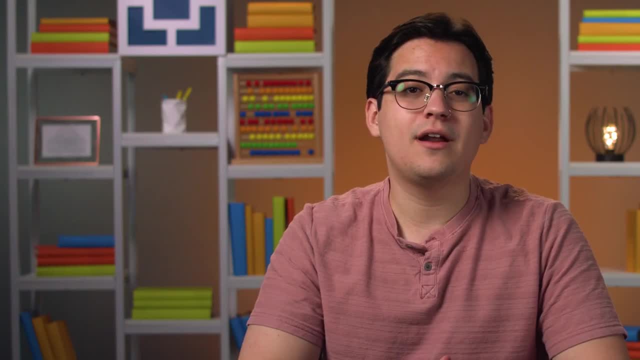 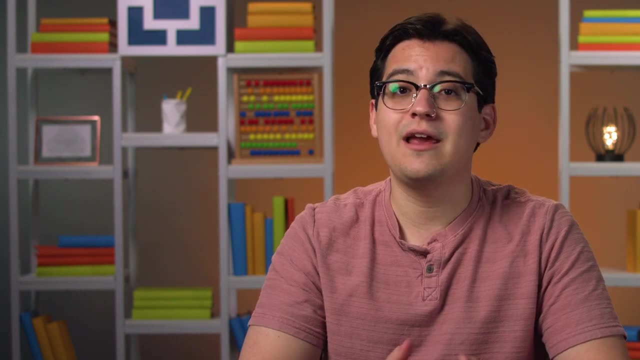 The more you start looking at things through a math lens, the more you can untangle complex patterns of information, solve problems or even admire the hidden structures and logic buried everywhere. But it's not always obvious how to do that right away. No need to fear, though, In math. 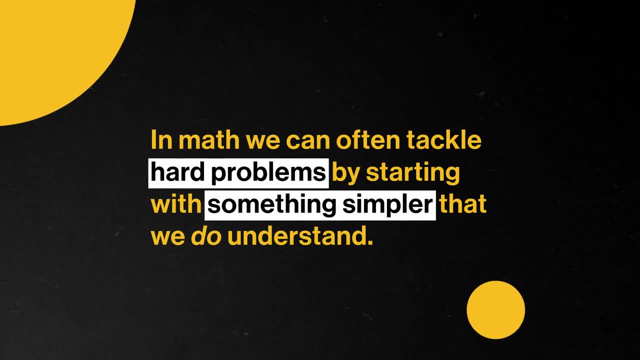 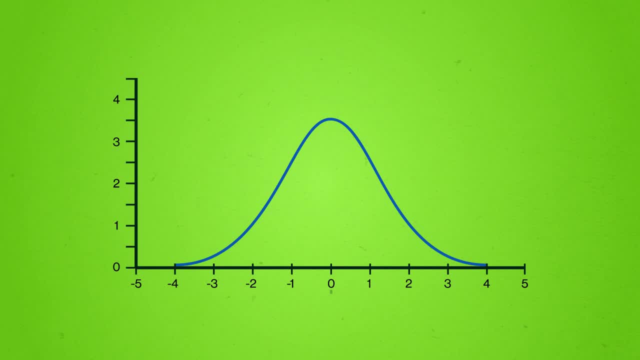 we can often tackle hard problems by starting with something simpler that we do understand. For instance, let's explore that bell-shaped pattern we mentioned in the intro and why they show up so often. They might look familiar, since last episode we talked about normal. 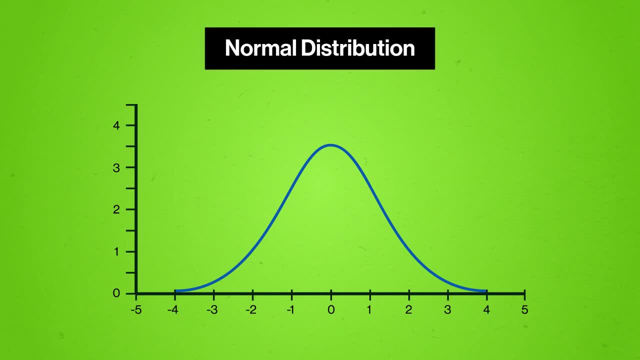 distributions, which is what we call data. that gives us a particular bell-shaped curve when we plot it, based on frequency. This bell-shaped curve also tells us about probabilities, which we'll get into more in a second, And it's defined by two numbers: a mean and a standard deviation. 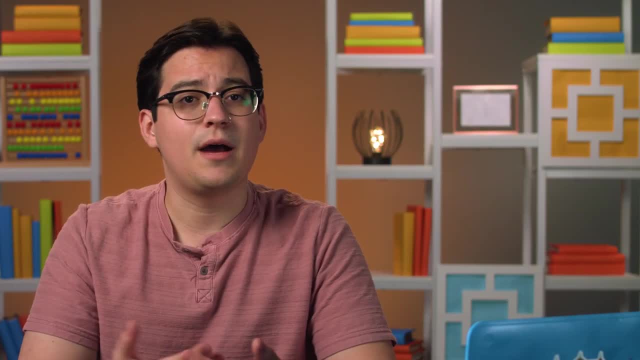 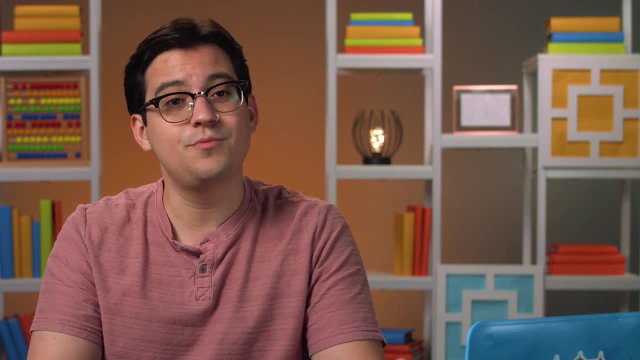 Like, say you were recording the body weights of newborns in a population which doctors and public health professionals look at to study the health of babies? Birth weights broadly follow a normal distribution And in the US that distribution for babies born at term has a mean of 3.4 kilograms and 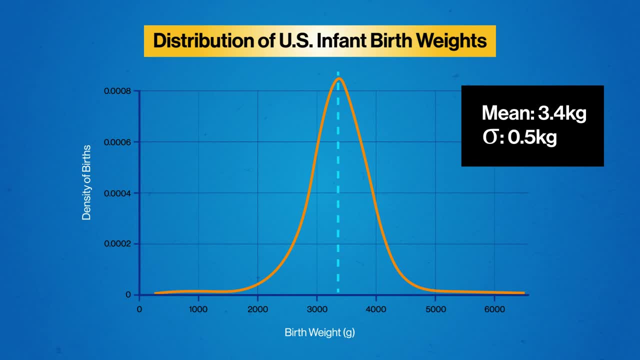 a standard deviation of half a kilogram. The mean tells us where the center of the distribution is, and in this case the average weight of a baby, And the standard deviation tells how spread out the data is around that center, which in this case is broadly how much we expect weight to vary between newborns. 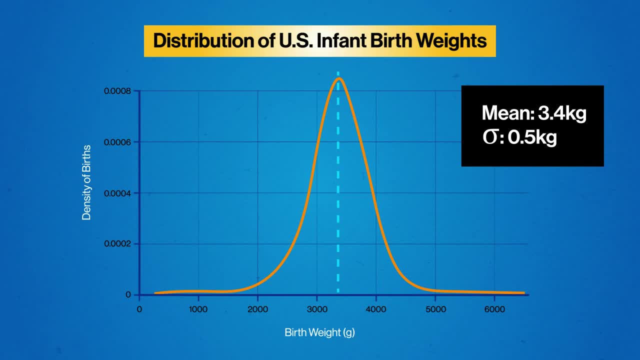 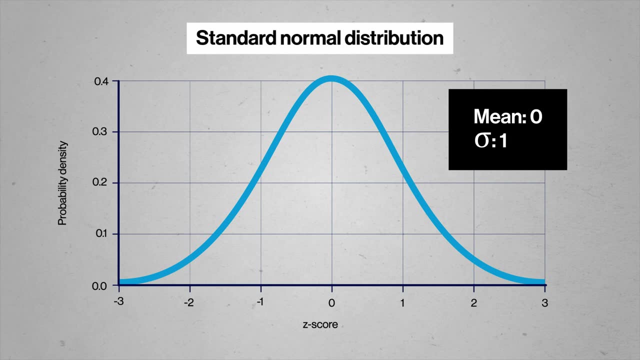 So both the mean and the standard deviation affect the shape of our curve. Last episode we focused on a particular normal distribution called the standard normal curve, where the mean is 0 and the standard deviation is 1.. And, as we learned, we know a lot about. 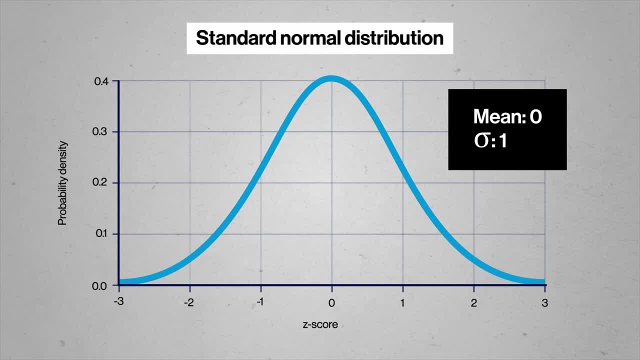 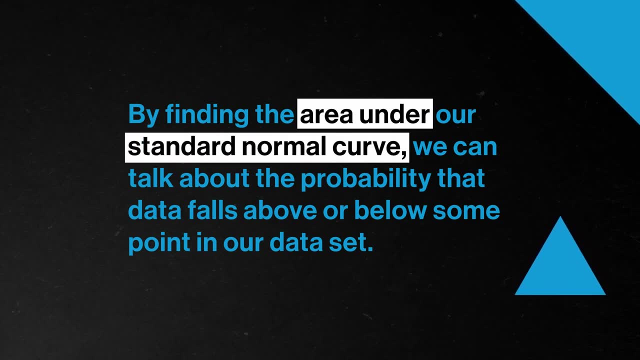 standard normal curves so we can use them to work with all the other normal curves we might find Like. by finding the area under our standard normal curve, we can talk about the probability that data falls above or below some point in our data set. We do this using z-scores. 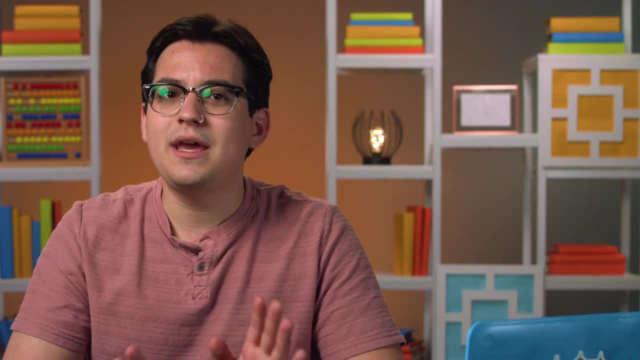 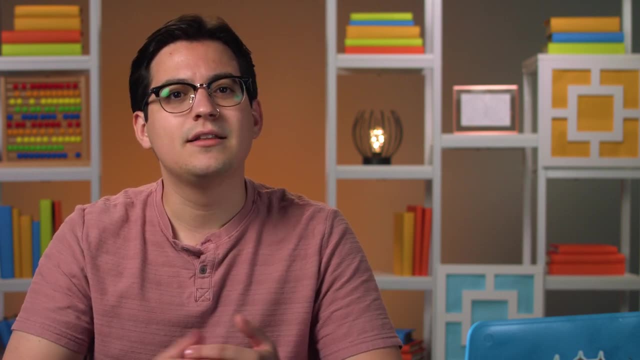 which we talked about last episode. Check out that episode for a refresher. But basically a z-score tells us how many standard deviations a particular point is from the center of the data set, Like in a data set about the weights of newborns. 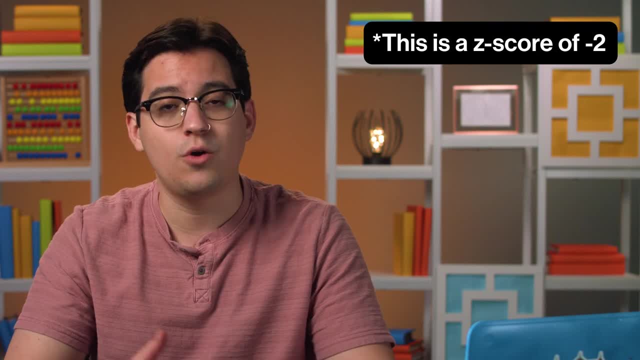 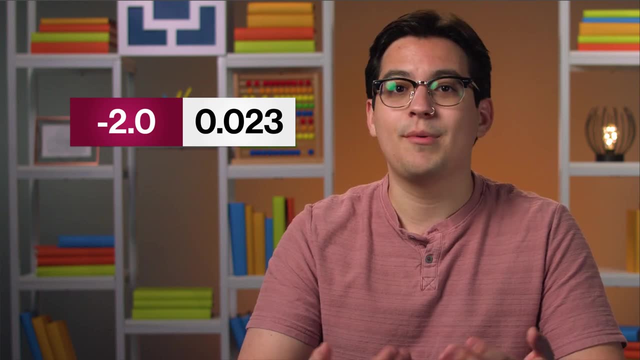 and how many babies have a weight less than 2 standard deviations below the mean. We can look up that z-score in a z-score table to figure out the area under the curve up to that point which gives us the probability. So if we look up negative 2 in a z-score table, 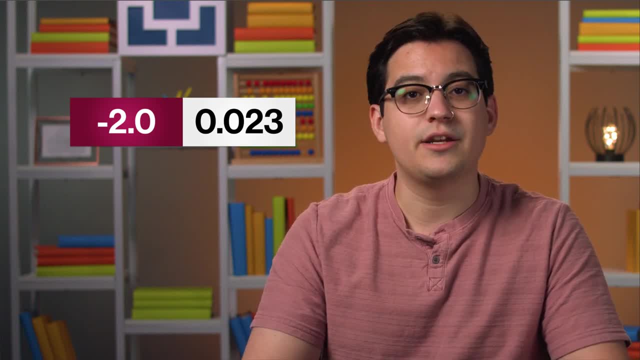 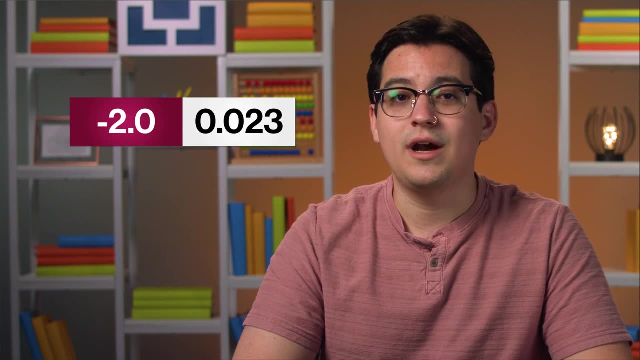 that tells us the area under the curve to the left of that point, we'd get 2.3%, And that means there's about a 2.3% probability of any given newborn in the US weighing LESS than whatever weight is two standard deviations below the mean. All of this is 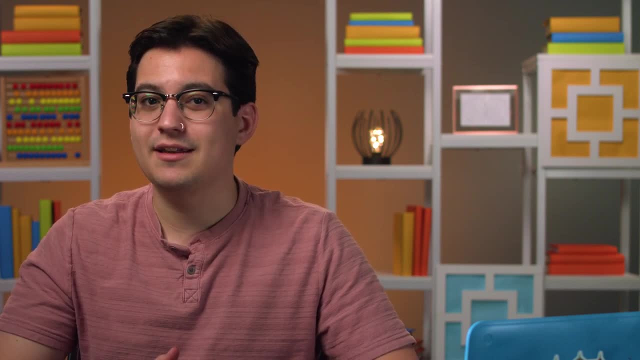 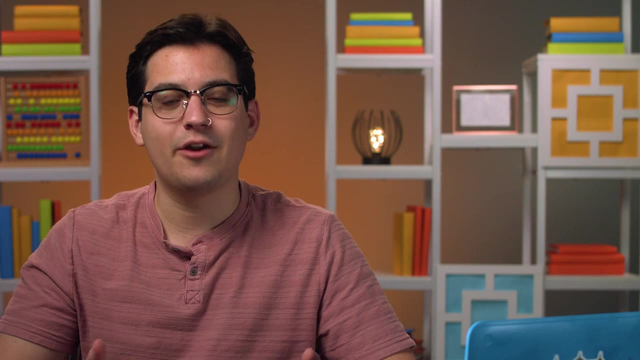 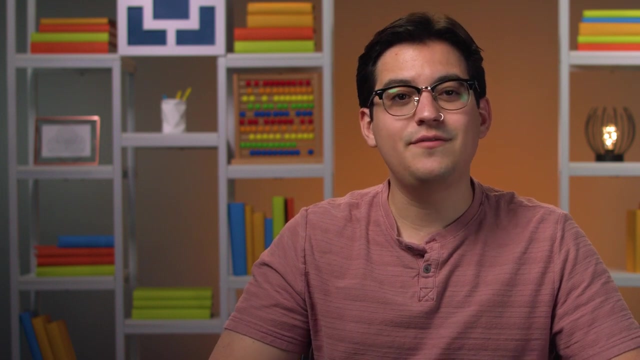 pretty important because when we're looking at distributions and the shape of a data set, figuring out how likely a point is to be in our set or how likely something is to happen, is a big part of why we care about distributions at all. Unfortunately, to use z-scores, we need to know about standard deviations And the standard. 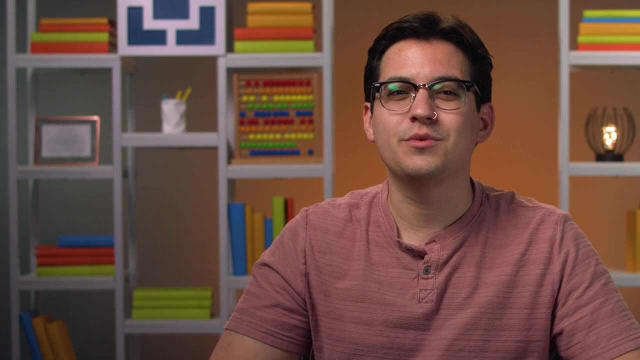 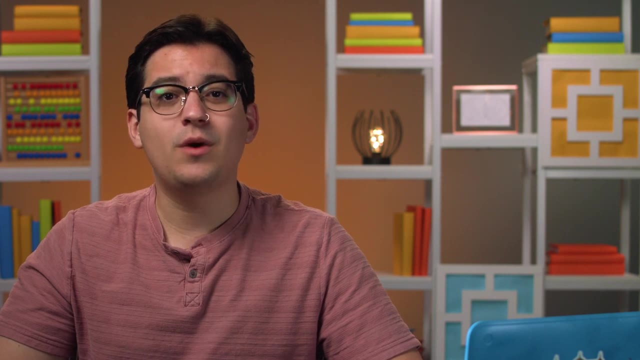 deviation of a data point isn't as obvious when we're not working with a standard, normal curve, which is… most of the time Like. rather than talking in terms of standard deviations, we might want to know something like… How many babies are born with a weight less than two and a half kilograms? 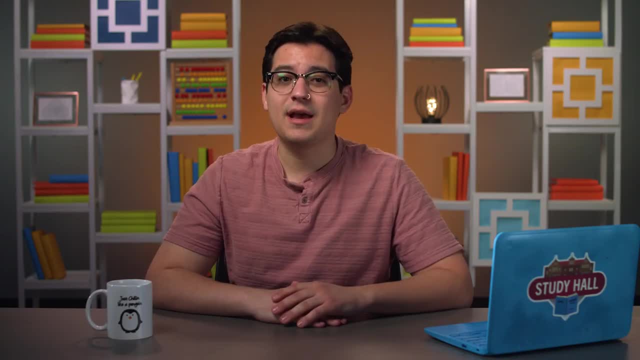 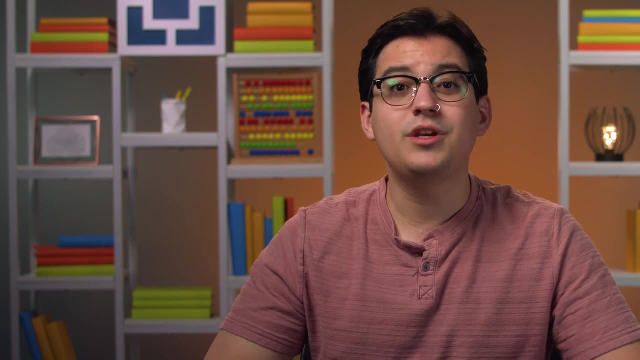 To answer questions like these, we need a way to connect our idealized math world to the kinds of distributions we'll find out in the wild. Fortunately, in math, when we're trying to solve a complicated problem, we can use what we already know about a simpler case, And it turns out we can adjust the standard. 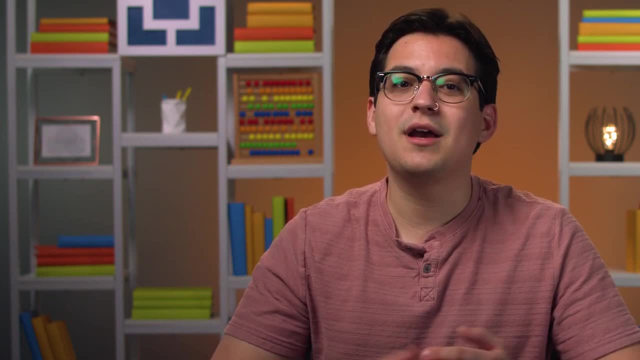 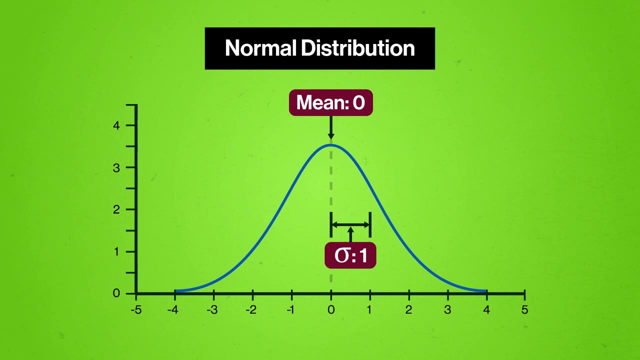 normal curve in order to find z-scores and make exactly the same kinds of probability calculations for any normal distribution we find in the wild. It's actually fairly simple to adjust bell-shaped curves Depending on our new mean- we can move it around the x-axis- And depending on our standard. 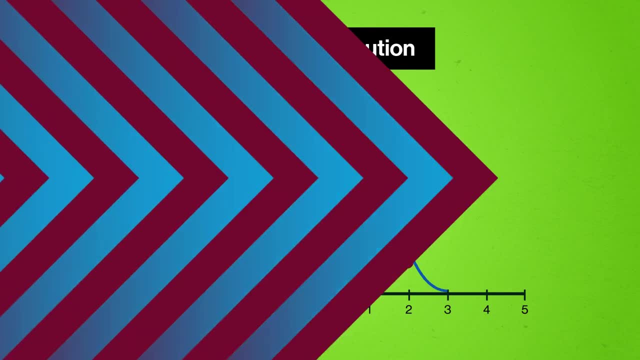 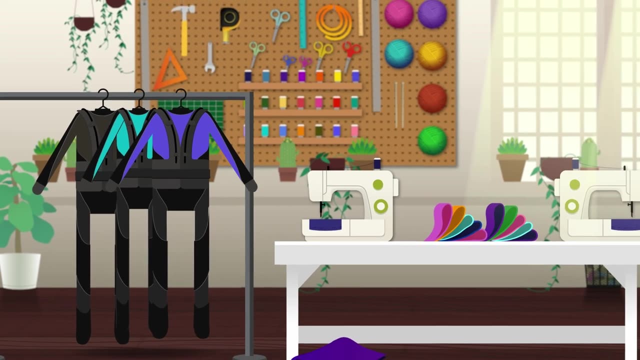 deviation. we can stretch or squeeze it to fit our data. To see how we do that, let's check out custom wetsuit designer Aria, who's trying to forecast the costs for running her new business. Aria's wetsuits are tailor-made to size. From taking measurements, she can estimate. 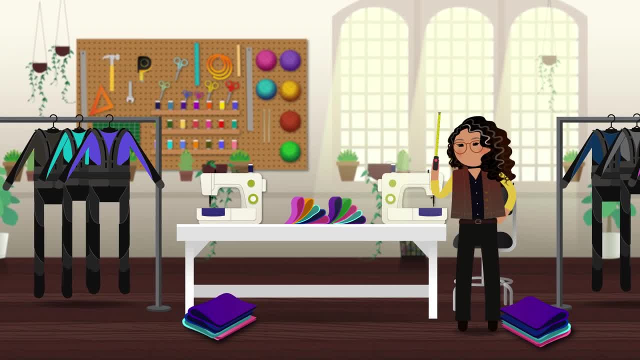 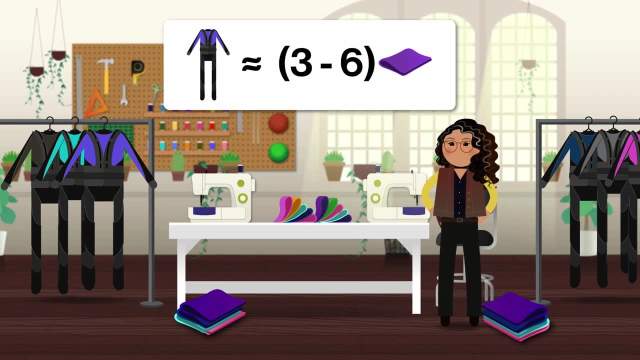 the surface area of a customer's body which tells her how many sheets of neoprene she needs for each order. A suit usually requires between three to six sheets of neoprene, but she can't order it in a single order. She can't order in bulk ahead of time because each customer has different requests for how thick the material is, style and color. 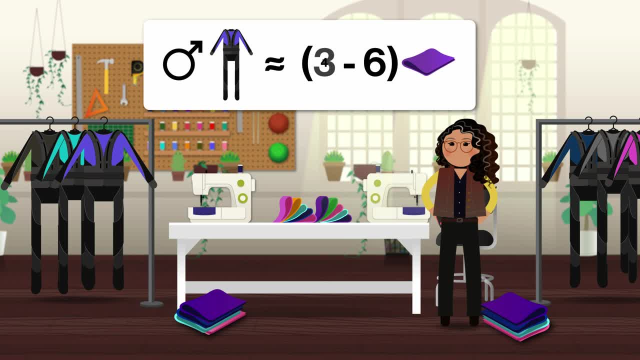 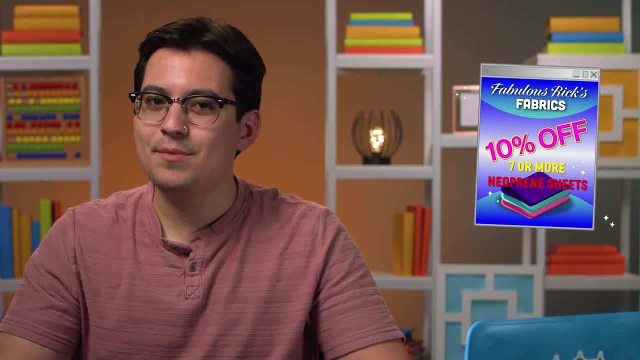 They are bespoke after all. On average, her male customers tend to be a bit larger and occasionally she finds that some of them require at least seven whole sheets to make a suit. And, as it happens, her supplier just announced they'll offer a discount when ordering seven. 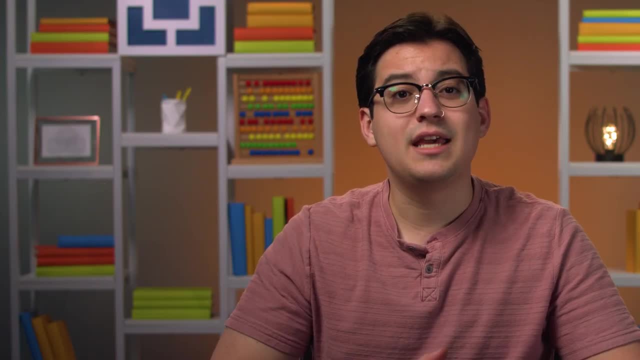 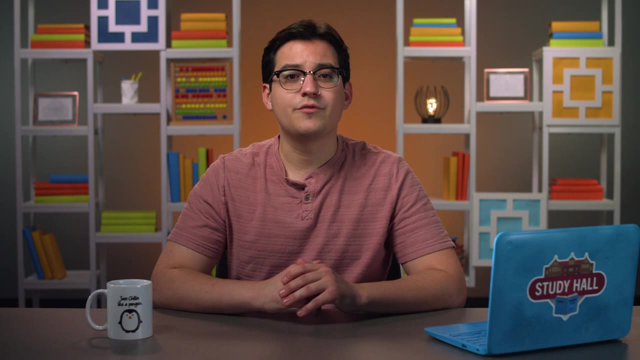 or more sheets. So Aria wants to know how often she'll get this discount on her neoprene orders for male customers. In advance of this, we need a couple of details from Aria's records of her previous customers. First of all, we need to know how much material she used for each of her previous wetsuit orders. 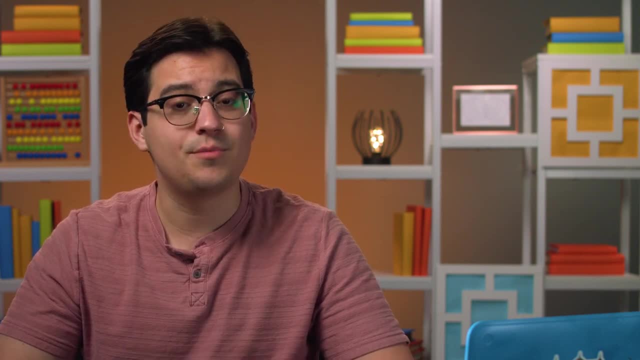 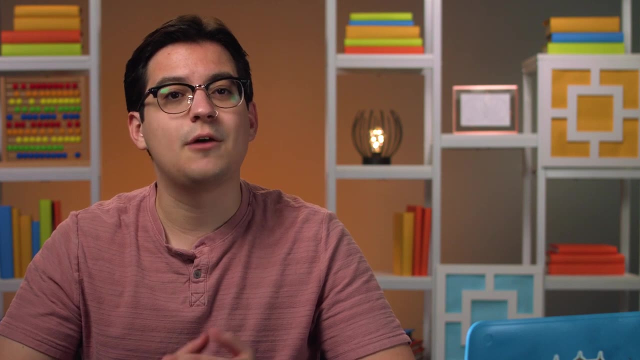 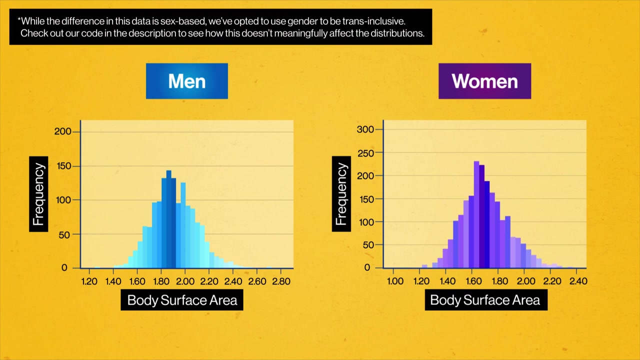 which depends on the body sizes of different customers and how that data is distributed. She doesn't have a ton of historical data, so for the most accurate probabilities, she also looks up information on how people's body shapes are distributed. As it turns out, we've studied it a lot and for a given gender, the surface area of 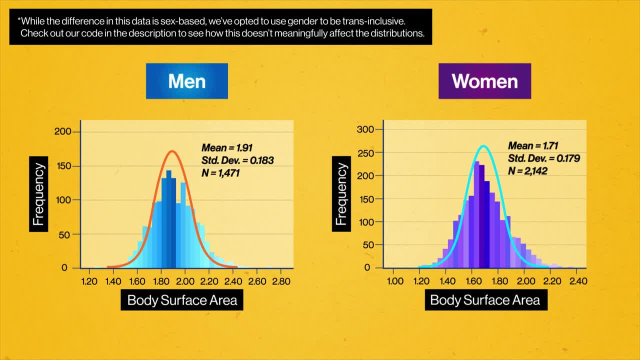 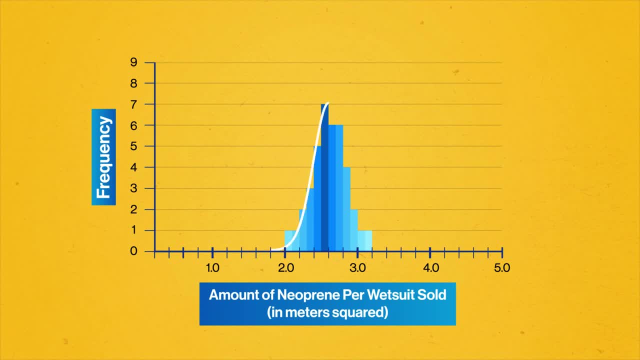 human bodies follows. hey, what do you know? And since the material for each wetsuit depends on the size of the person, the amount of material she's used for each suit also follows a normal distribution. From her customer records, the distribution of the neoprene has a mean of 2.6 meters squared. 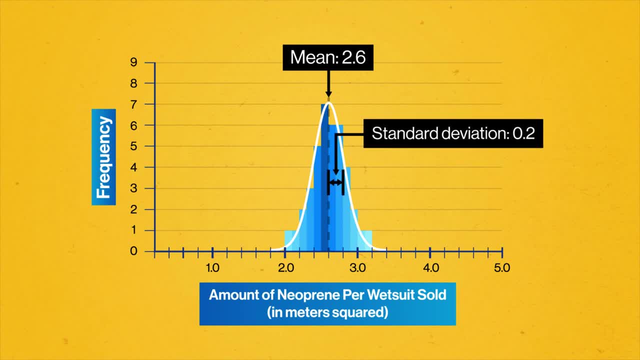 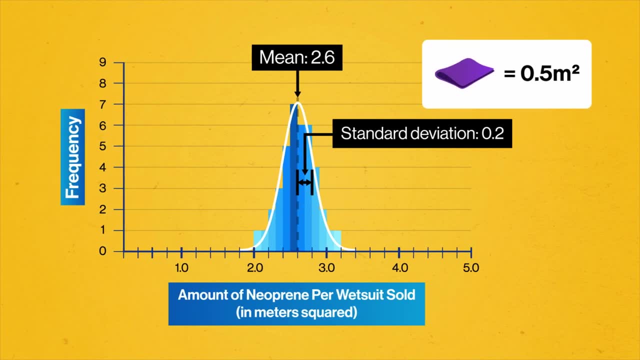 and a standard deviation of 0.2 meters squared. We then need to know how the amount of neoprene corresponds to the number of sheets Aria orders. Well, the sheets come in units of half a meter squared, so if a customer needs more than, 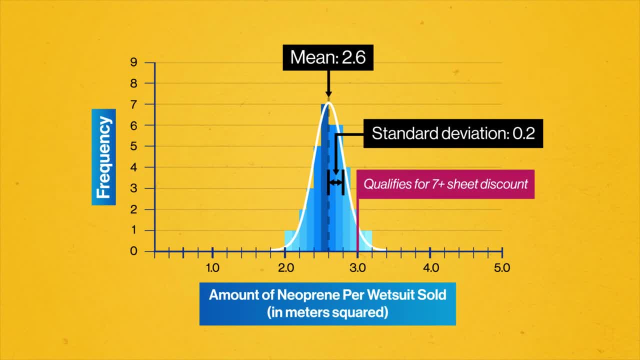 three meters squared, it takes seven or more sheets. So now that she knows that the amount of neoprene she orders is normally distributed and that any order that needs three square meters or more qualifies for the discount, she can use that information, plus the power of z-scores, to figure out how likely it is. 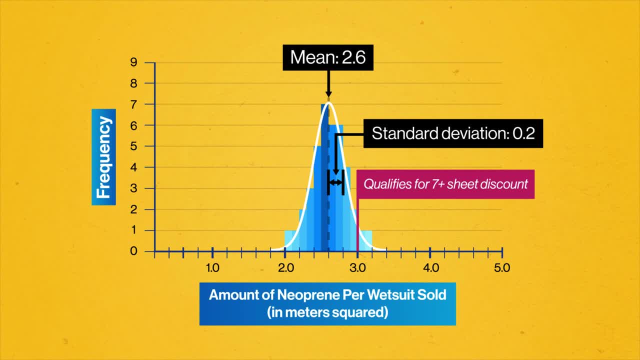 an order will qualify for the discount. Basically, Aria will calculate the area under the curve to the right of three on the x-axis. That will give her the probability. an order needs three square meters or more of neoprene, which are all orders where she gets the bulk. 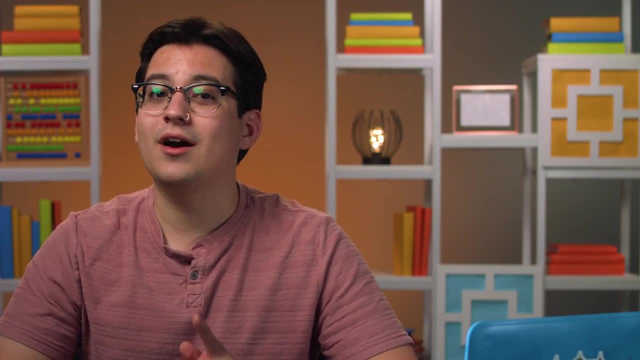 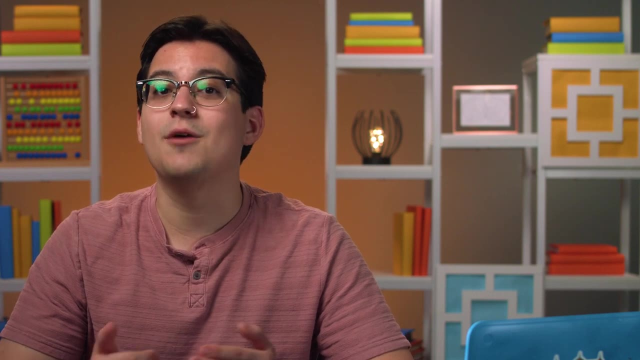 Now comes the clever part. Remember, on the standard normal curve, where a data point is along the x-axis is the same as how many standard deviations it is above or below the mean. So by transforming our normal curve into a standard normal curve we can find how many. 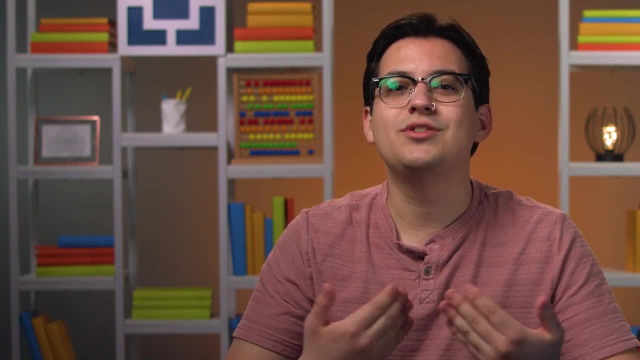 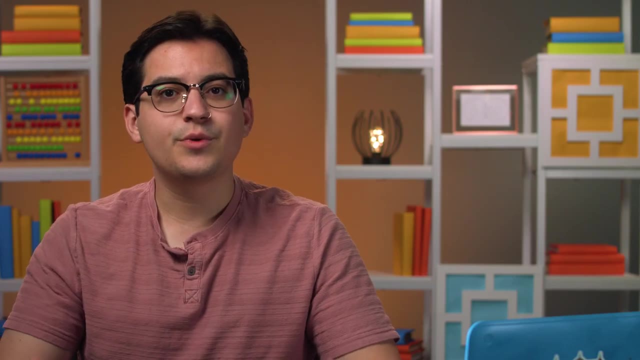 standard deviations. each point is away from the mean, which is exactly how we define z-scores, And then we can use that to calculate the area under the curve. In particular, since we're looking for people with body sizes three minus one, we can use z-scores to calculate the area under the curve. In particular, since we're looking for people with body sizes three minus one, we can use z-scores to calculate the area under the curve. Since we're looking for people with body sizes three minus one, we can use z-scores to calculate the area under the curve. 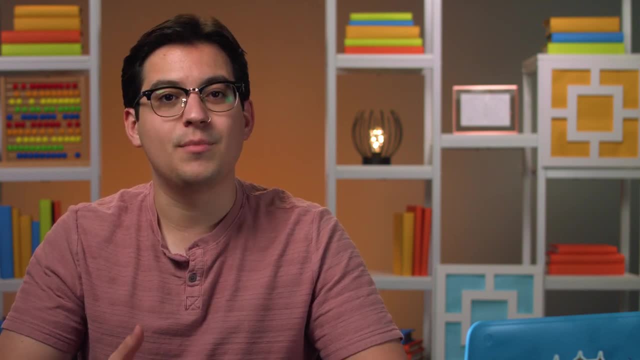 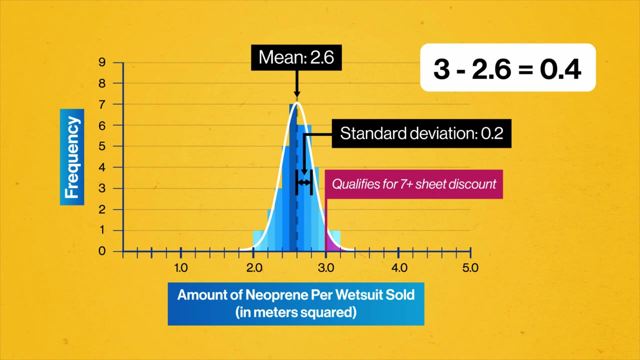 To do this, we can work out how many standard deviations. three is above the mean. First we need to subtract the mean from the point we're interested in to get the distance between the two numbers. If we do this in general for the entire curve, we could write it using statistical notation. 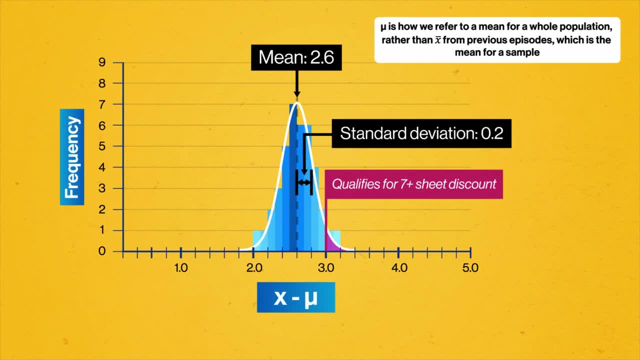 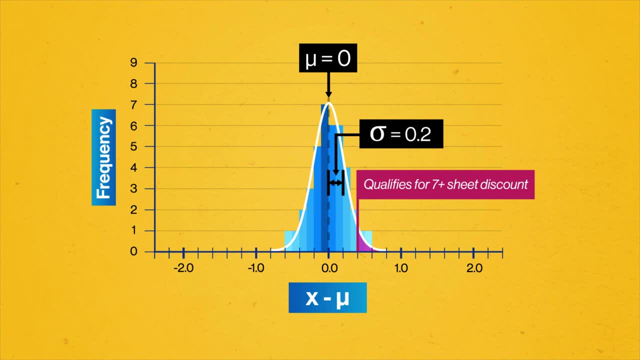 and call our mean mu and our particular value x. Doing this shifts our whole distribution and re-centers it on 0.. Things are already looking closer to our standard normal curve. only the spread of the distribution isn't quite right. Right now our standard deviation is still 0.2, but we need to make 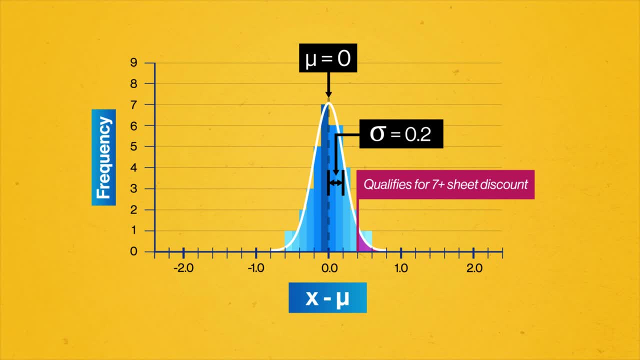 some adjustments to make it 1. if we want to find our z-score, To see how let's look at where the point that used to correspond to 3 square meters landed on this new distribution. After subtracting the mean, it winds up at 0.4.. And to figure: 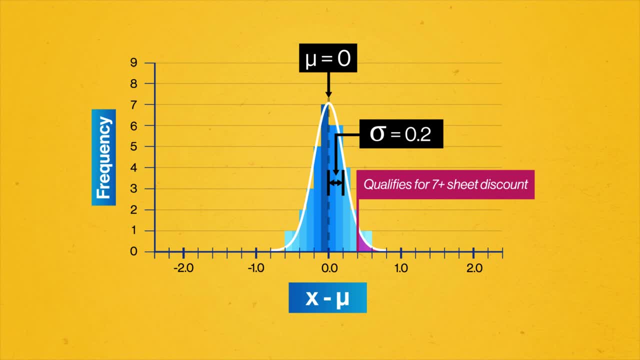 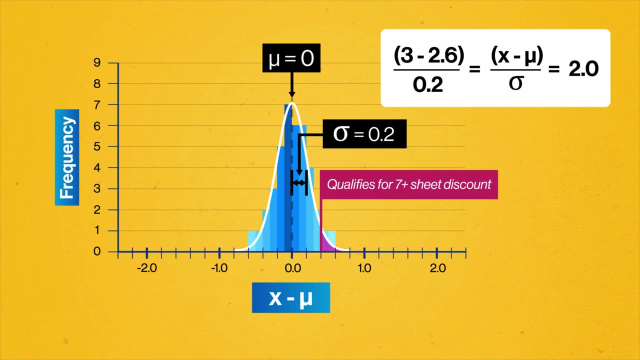 out how many standard deviations. that is away from 0, our new center. we simply divide everything by our standard deviation. It's like seeing how many 0.2 segments will fit between the mean and our data point and that will expand our data to fit the standard normal curve. 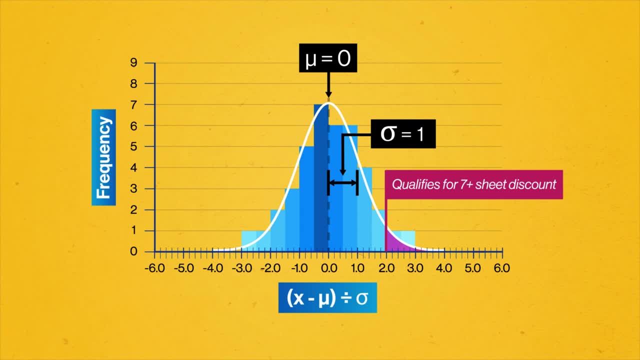 by stretching out all the points from the center. Now we've transformed our curve into the standard normal curve and we know that our point is two standard deviations away from the mean, And that's also exactly the same information we use when calculating z-scores. 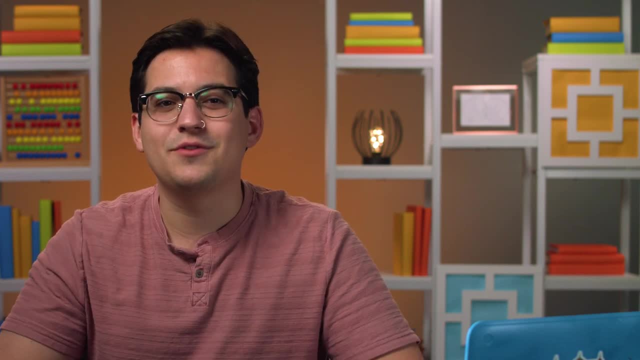 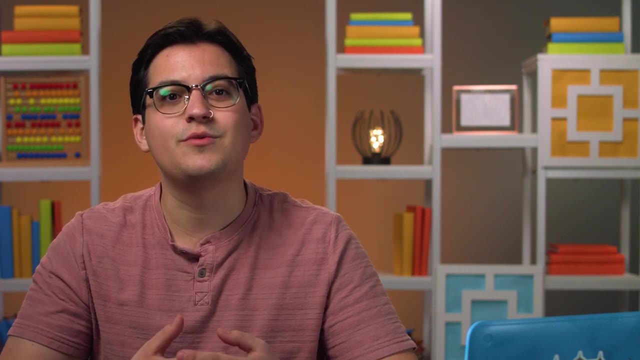 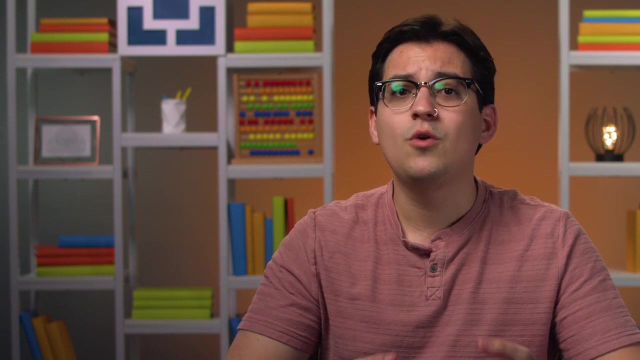 So here's the great thing: The probabilities we calculate for the standard normal curve are the same as the probabilities we calculate for the standard normal curve. So, to sum up, when we start off with some variable or data that follows a normal distribution, 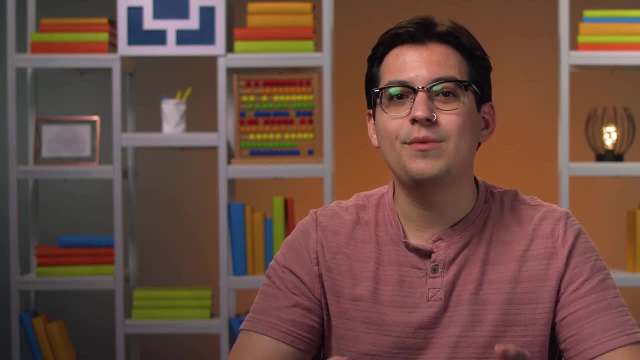 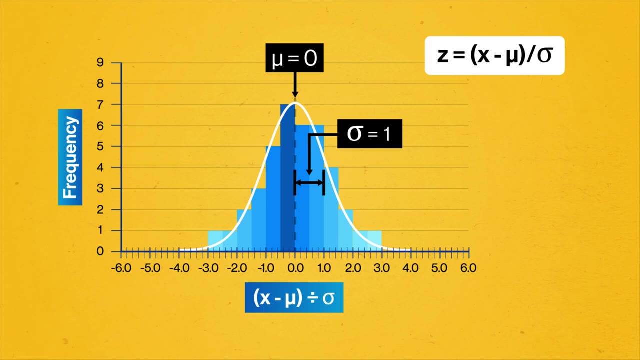 we can get the z-score for every possible value by transforming our normal distribution curve into the standard normal curve. We do that by subtracting the mean and dividing through by the standard deviation, In Arya's case to get the probability of needing more than 3 meters squared of neoprene. 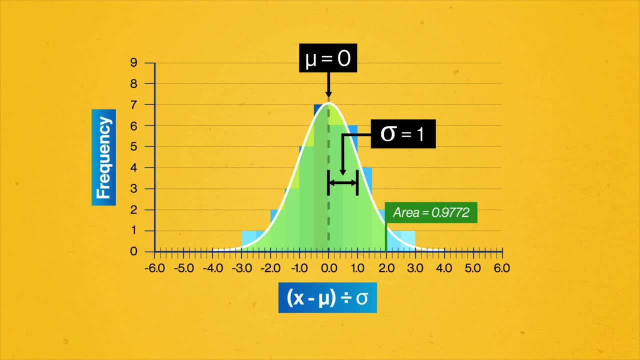 she looks up the z-score probability for 2.0 in a z-score table. Because of how the left of the tail table is set up, that gives her the probability of someone needing less than 3 square meters. So she then subtracts that number from 1,, since she wants the probability. 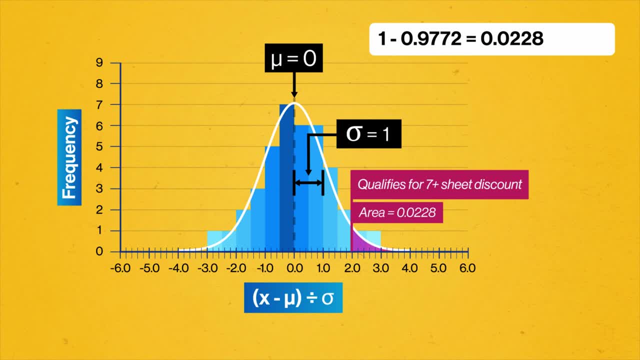 under the curve from the right of that point where all the values are larger than 3 meters squared. That gives her a probability of just over 2%. So that means she can expect to get a discount on neoprene for about… 1 in every 1.. 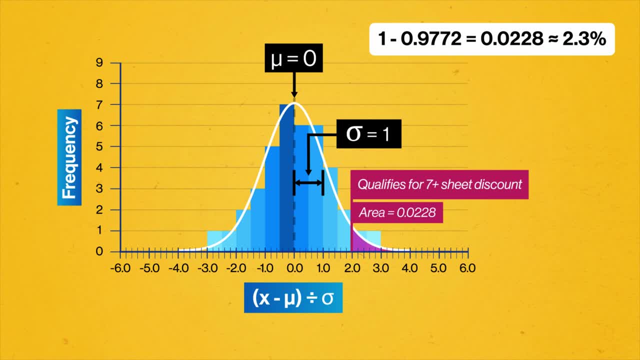 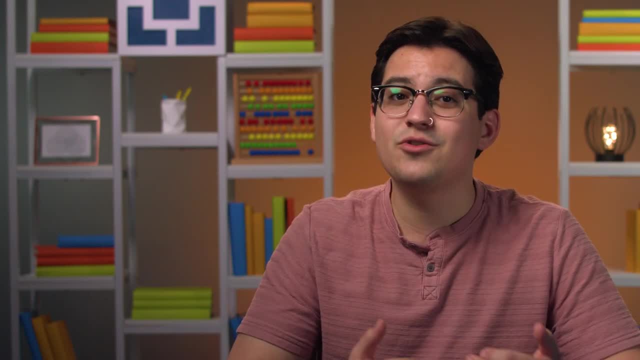 1 in every 50 orders, And with that knowledge she can plan her operating costs for her new business. In general, the ability to change between any arbitrary normal curve and the standard normal curve gives us a kind of mathematical bridge for calculating probabilities about. 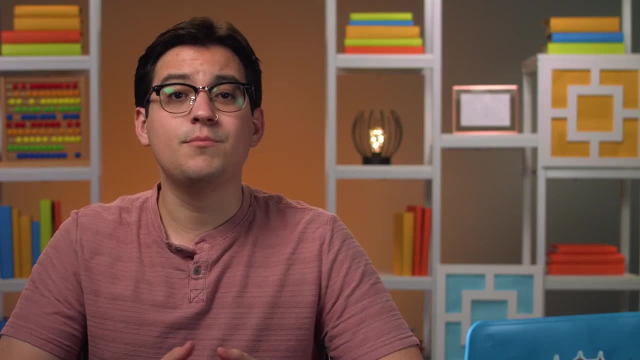 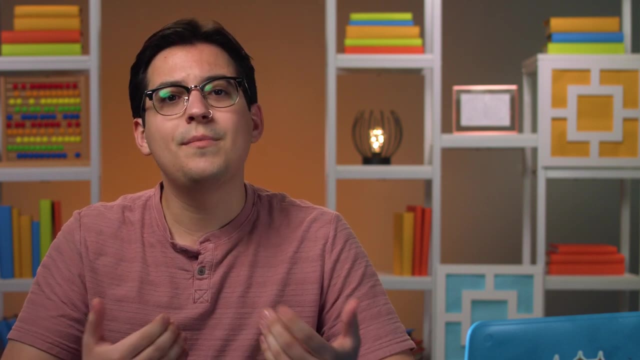 any normal distribution we come across When we subtract the mean to move the graph up and down the x-axis or divide through by the standard deviation to stretch or squeeze our data, we're manipulating our graph to fit our standard normal curve. This makes 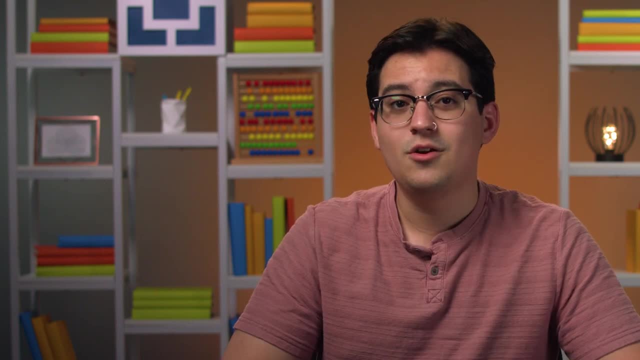 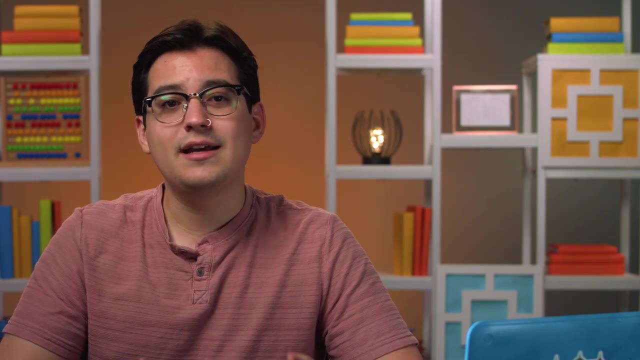 it easy to see why the standard normal curve is called standard. We can use our formula to map a normal distribution onto it and then use z-scores to calculate things about them. How body size affects business forecasts is just one example that highlights the power. 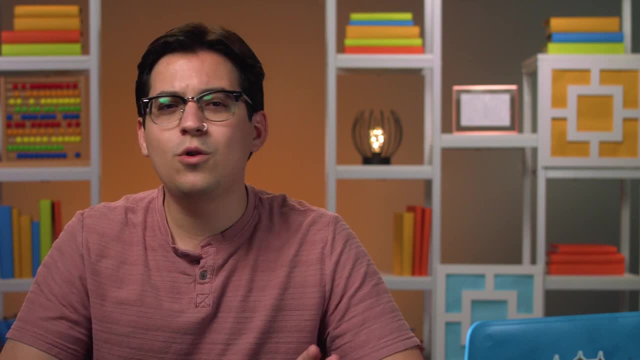 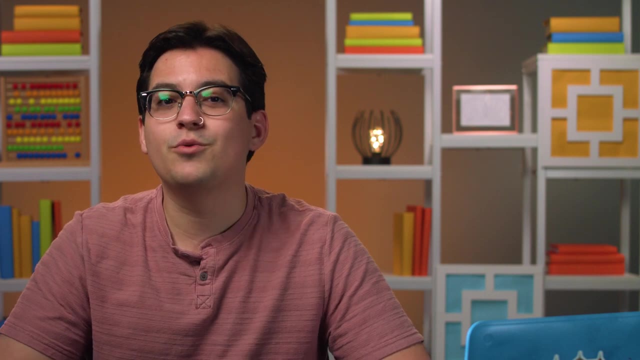 of statistics. Normal distributions pop up all over the place, from measurement errors in physics to other factors about people's body shapes and even test scores. But with the right math tools we can make sense of them all. Overall, the statistics and probability.